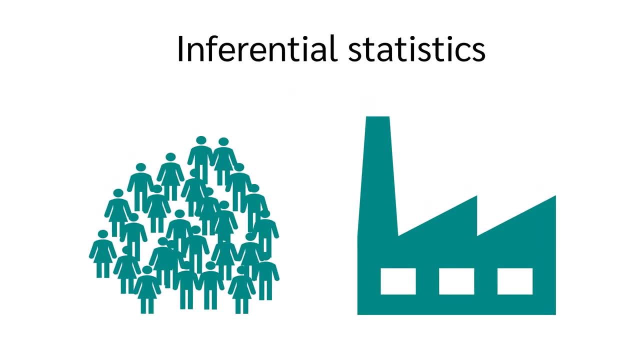 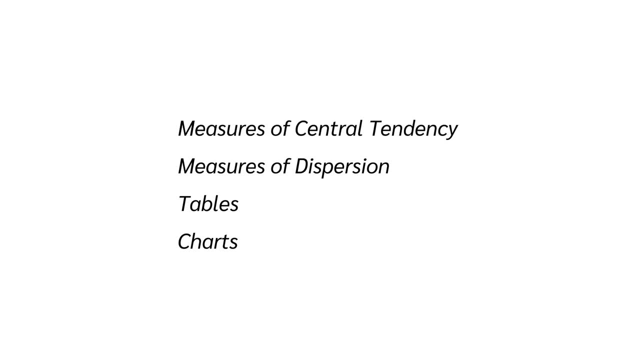 of the company get to work. This is the task of inferential statistics: To describe data descriptively. we now look at the four key components: Measures of Central Tendency, Measures of Dispersion, Frequency Tables and Charts. Let's start with the first one: Measures of Central Tendency. 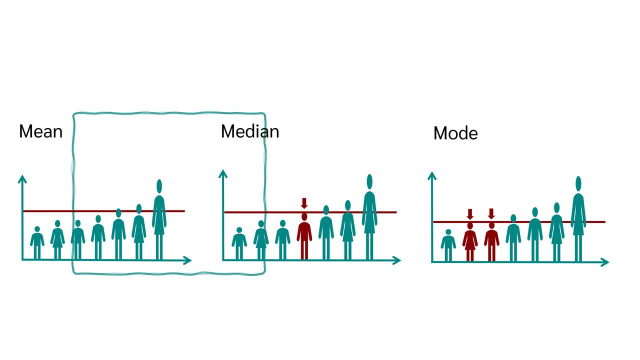 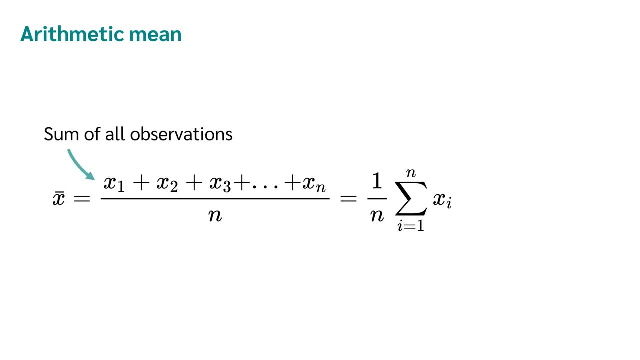 Measures of Central Tendency are, for example, the mean, the median and the mode. Let's first have a look at the mean. The arithmetic mean is the sum of all observations divided by the number of observations. An example: Imagine we have the test scores of five students To find 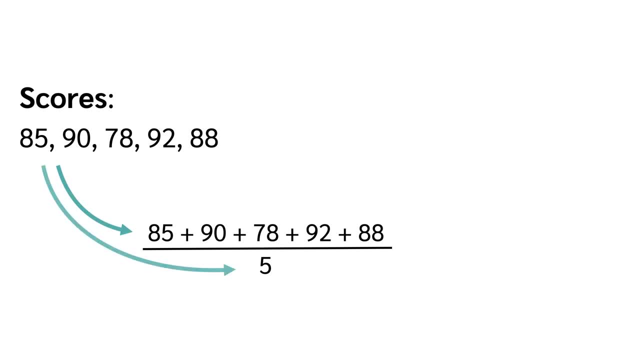 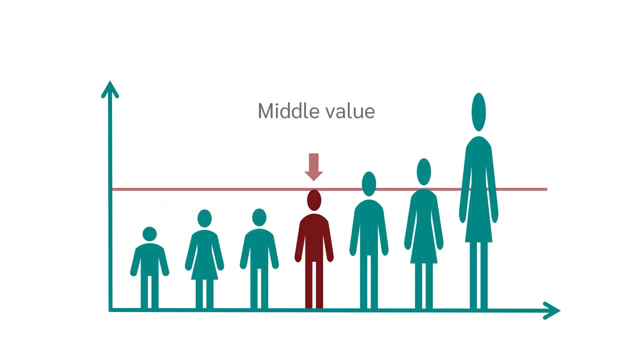 the mean score. we sum up all the scores and divide by the number of scores. The mean test score of these five students is therefore 86.6.. What about the median? When the values in a data set are arranged in ascending order, the median is the middle value, If there is. 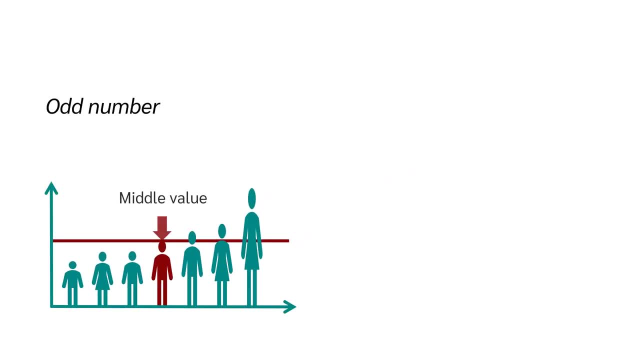 an odd number of data points, the median is simply the middle value. If there is an even number of data points, the median is the average value. The median is the average of the two middle values. It is important to note that the median 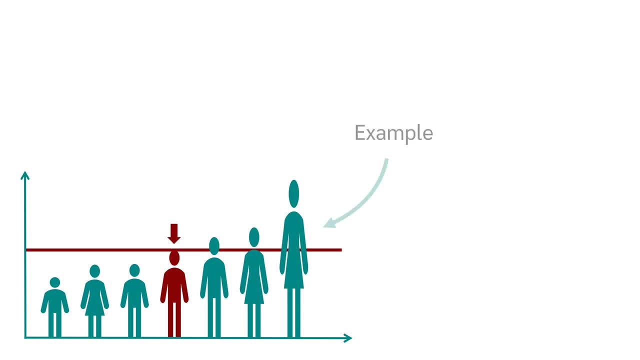 is resistant to extreme values or outliers. Let's look at this example. No matter how tall the last person is, the person in the middle remains the person in the middle, So the median does not change. But if we look at the mean, it does have an effect on how. 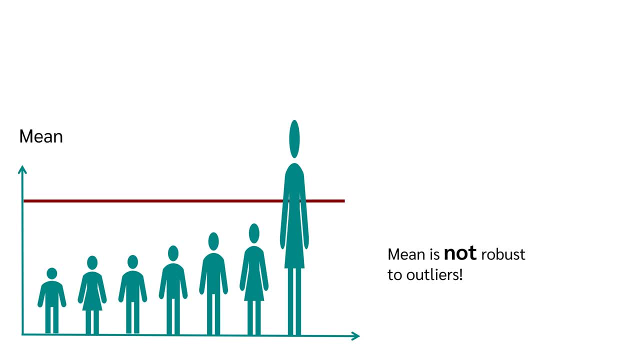 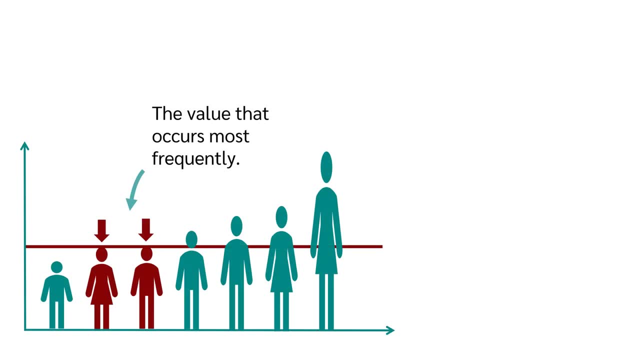 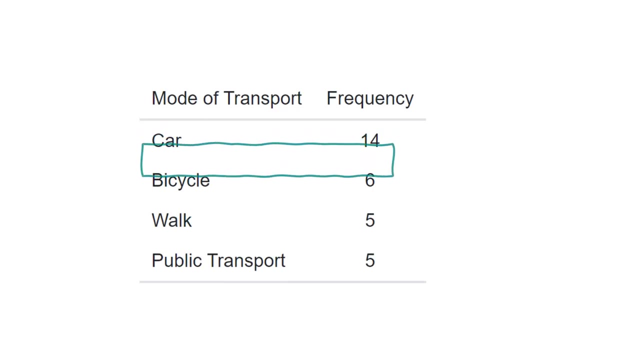 tall, the last person is. The mean is therefore not robust to outliers. Let's continue with the mode. The mode refers to the value or values that appear most frequently in a set of data. For example, if 14 people travel to work by car, 6 by bike, 5 walk and 5 take, 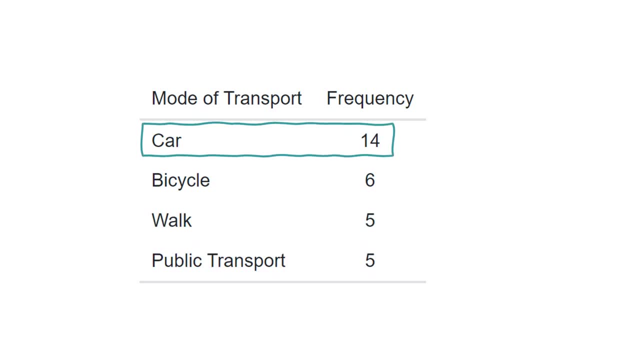 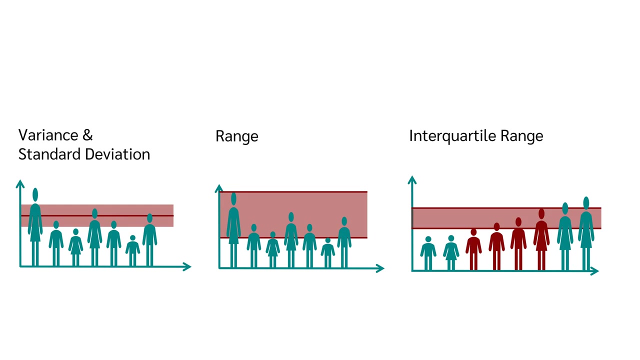 public transport, then car occurs most often and is therefore the mode. Great, let's continue with the measures of dispersion. Measures of dispersion describe how spread out the values in a data set are. Measures of dispersion are, for example, the variance and standard deviation, the range and the interquartile range. 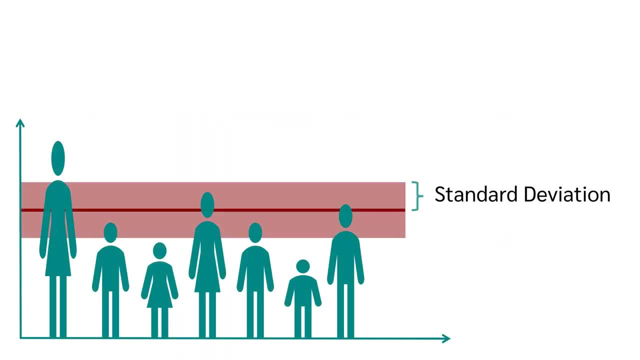 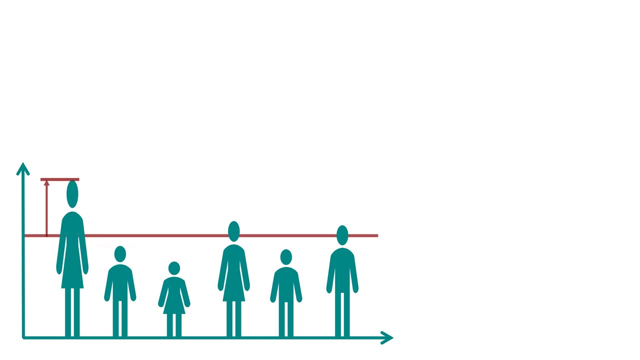 Let's start with the standard deviation. The standard deviation indicates the average distance between each data point and the mean. But what does that mean? Each person has some deviation from the mean. Now we want to know how much the persons deviate from the mean value. 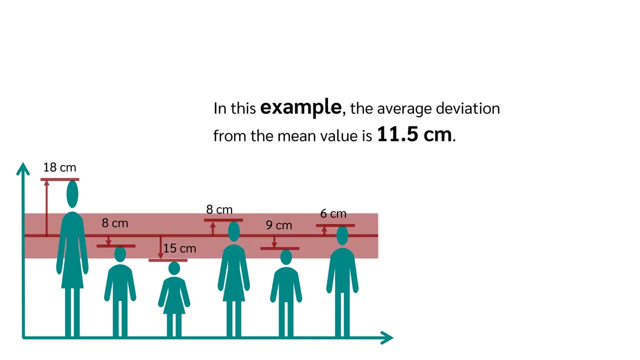 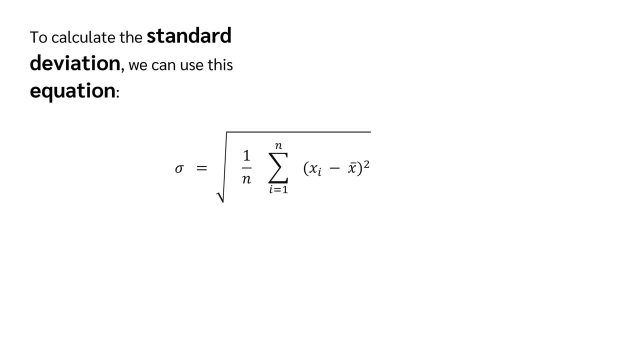 on the data set. Let's start with the standard deviation. The standard deviation indicates average. In this example, the average deviation from the mean value is 11.5 cm. To calculate the standard deviation, we can use this equation: Sigma is the standard deviation, n is the. 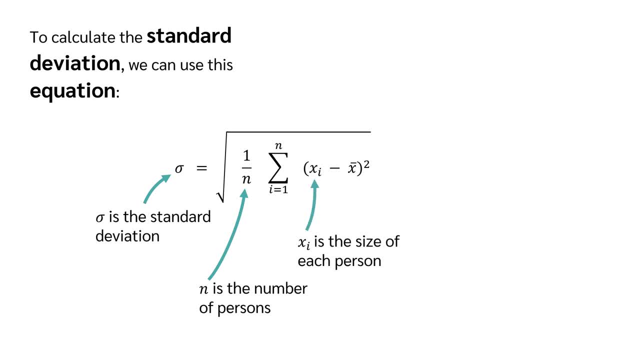 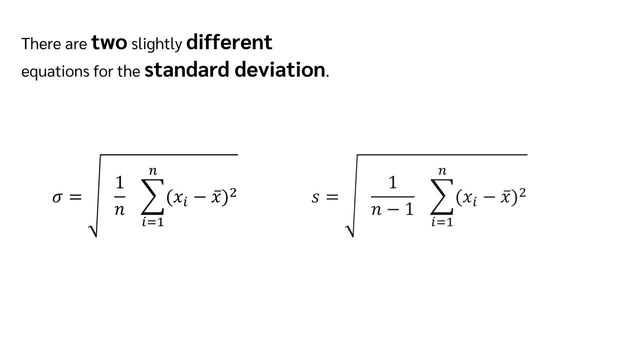 number of persons. xi is the size of each person and x-bar is the mean value of all persons. But attention, there are two slightly different equations for the standard deviation. The difference between the standard deviation and the average deviation is the number of persons. The difference is that we have once 1 divided by n and once 1 divided by n-1.. To keep 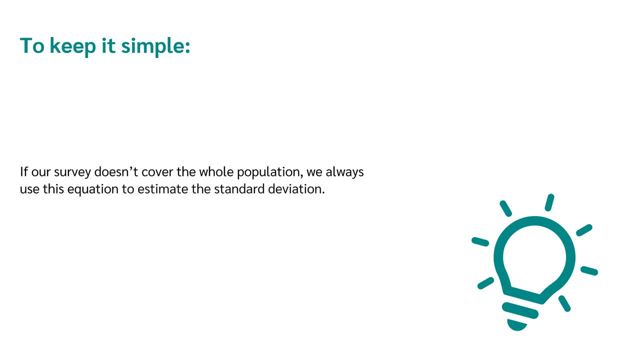 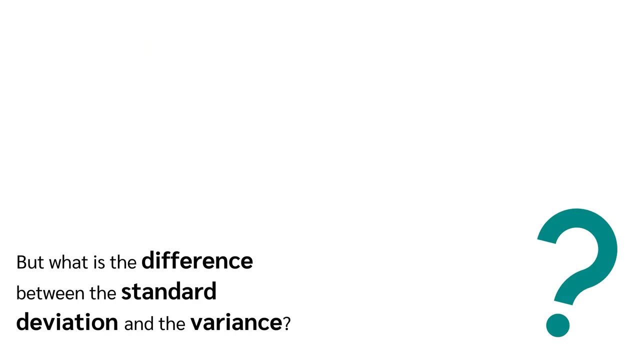 it simple: if our survey doesn't cover the whole population, we always use this equation to estimate the standard deviation. Likewise, if we have conducted a clinical study, then we also use this equation to estimate the standard deviation. But what is the difference between the standard? 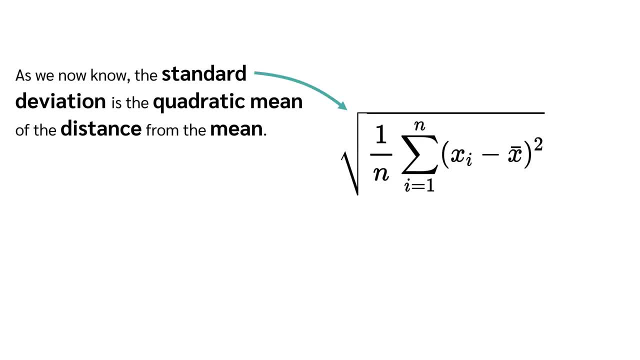 deviation and the variance. As we now know, the standard deviation is the number of persons. The variance now is the squared standard deviation. If you want to know more details about the standard deviation and the variance, please watch our video. Let's move on to range and interquartile range. It is easy to understand. The range is simply. 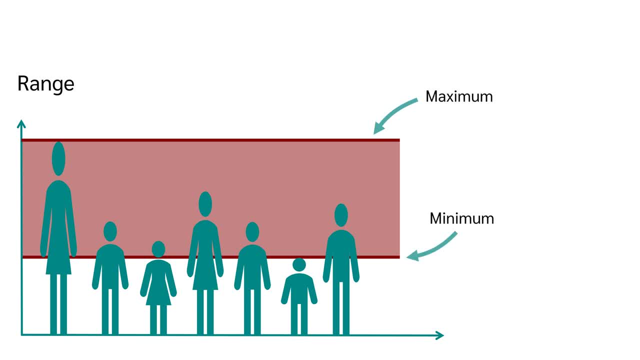 the difference between the maximum and minimum value. Interquartile range represents the middle 50% of the data. Interquartile range represents the maximum and minimum value. The range is simply the difference between the maximum and minimum value Interquartile. 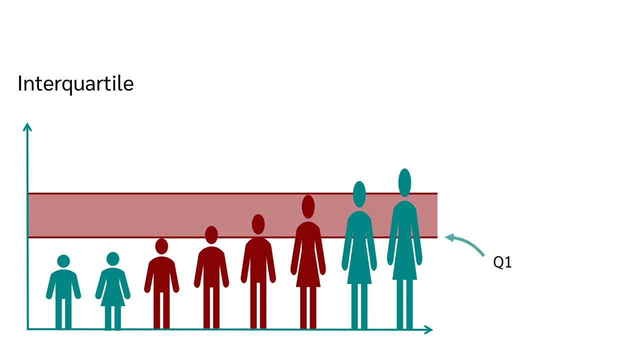 range represents the minimum and minimum value. The range is simply the difference between the first quartile and the third quartile. Therefore, 25% of the values are smaller than the interquartile range and 25% of the values are larger- The interquartile range. 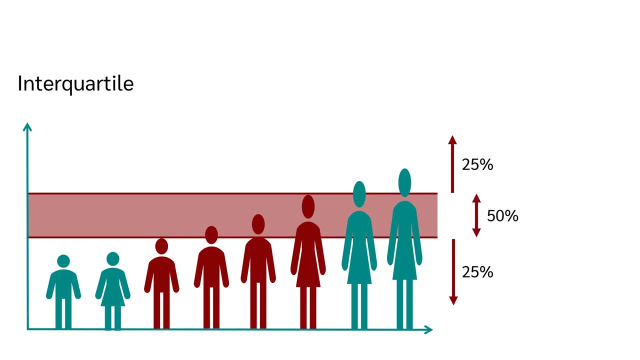 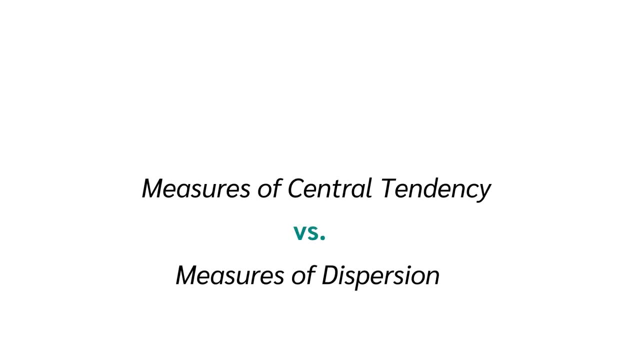 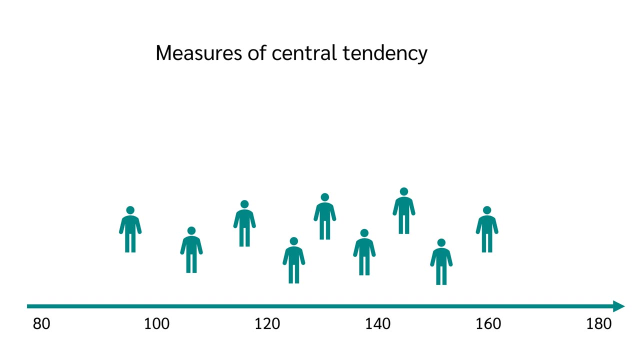 contains exactly the middle 50% of the values. Before we get to the last two points, let's briefly compare measures of central tendency and measures of dispersion. Let's say we measured the blood pressure of patients. Measures of central tendency provide a single value that represents the entire dataset, helping to identify a central value. 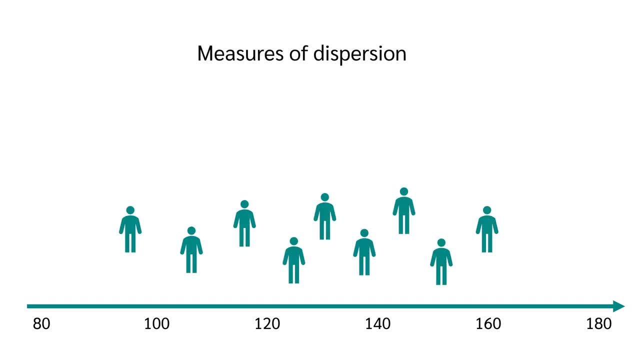 around which data points tend to cluster. Measures of dispersion, like the standard deviation, the range and the interquartile range indicate how spread out the data points are, whether they are closely packed around the center or spread far from it. In summary, while measures of central tendency provide a central point of the dataset, measures, 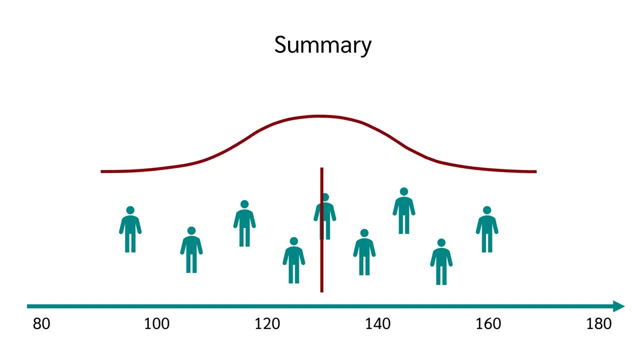 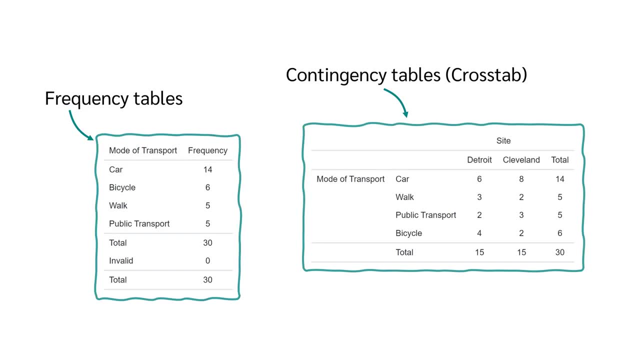 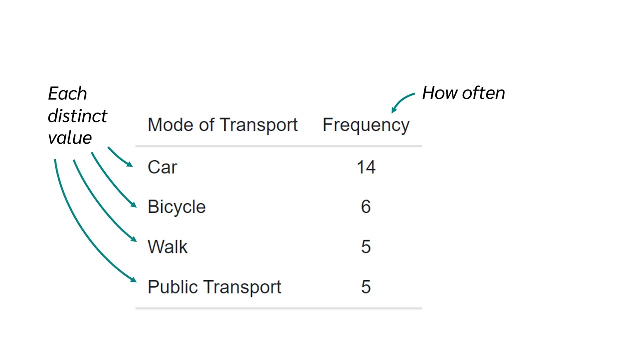 of dispersion describe how the data is spread around the center. Let's move on to tables. Here we will have a look at the most important ones: frequency tables and contingency tables. A frequency table displays how often each distinct value appears in a dataset. Let's have a closer look at the example from the beginning: A. 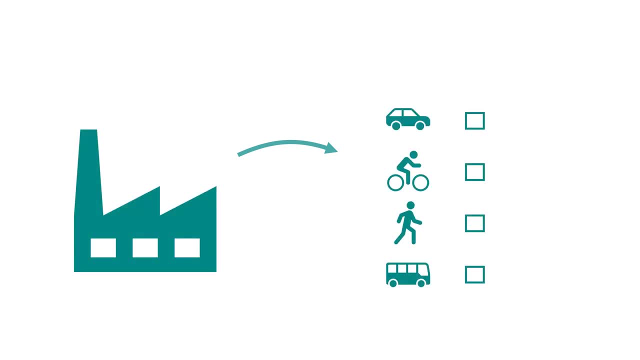 company surveyed its employees to find out how they get to work. The options given were car, bicycle, walk and public transport. Here are the results from 30 employees. The first answered car, the next walk, and so on and so forth. Now we can create a frequency table to summarize this data. 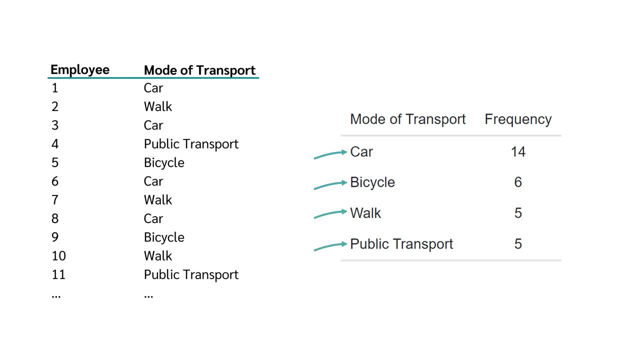 To do this, we simply enter the four possible options- car, bicycle, walk and public transport- and then count how often they occurred From the table. it is evident that the most common mode of transport among the employees is by car, with 14 employees preferring it. 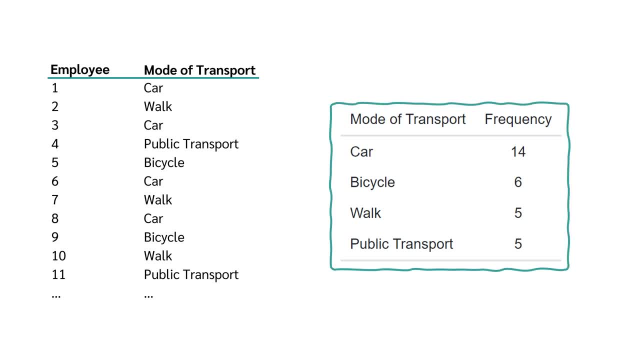 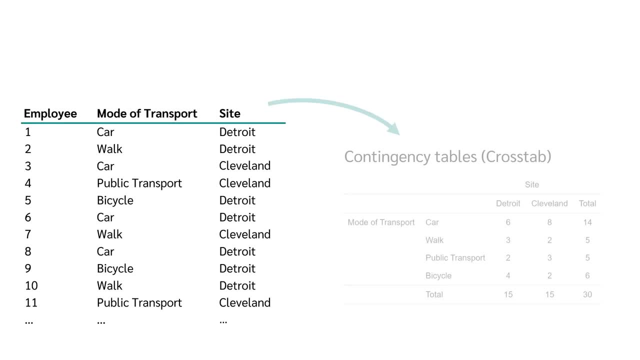 The frequency table thus provides a clear and concise summary of the data. But what if we have not only one, but two categorical variables? This is where the contingency table, also called crosstab, comes in. Imagine the company doesn't have one variable. 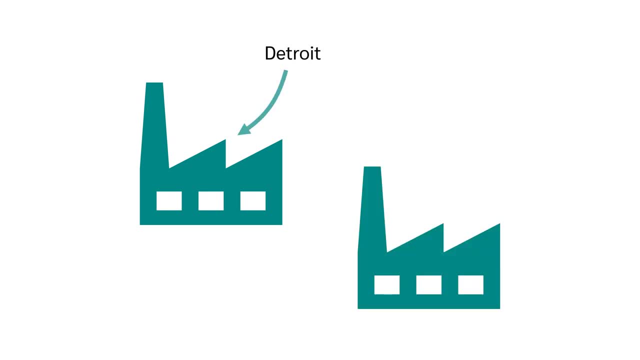 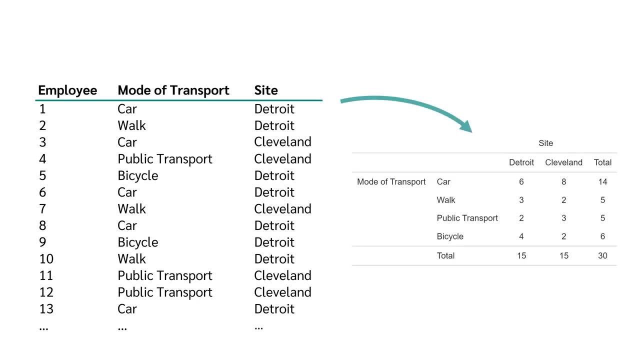 Imagine the company doesn't have one variable. Imagine the company doesn't have one variable. We have no factory, but two, One in Detroit and one in Cleveland. So we also ask the employees at which location they work. If we want to display both variables, we can use a contingency table. 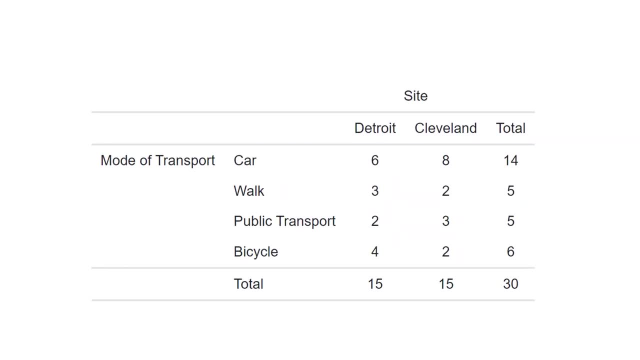 A contingency table provides a way to analyze and compare the relationship between two categorical variables. The rows of a contingency table represent the categories of one variable, while the columns represent the categories of other categories of another variable. Each cell in the table shows the number of observations that fall into the corresponding. 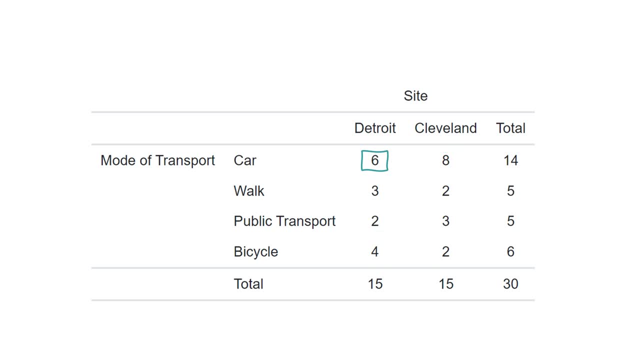 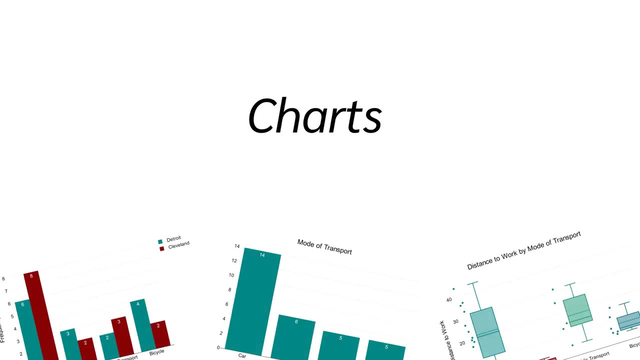 category combination. For example, the first cell shows that car and Detroit were answered 6 times. And what about the charts? Let's take a look at the most important ones. To do this, let's simply use datadepthnet. 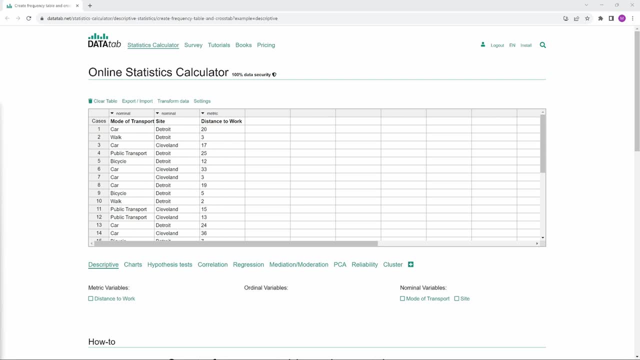 If you like, you can load this sample dataset with the link in the video description, Or you just copy your own data into this table. Here below you can see the variables: distance to work, mode of transport and site. Datadepth gives you a hint about the level of measurement, but you can also change it. 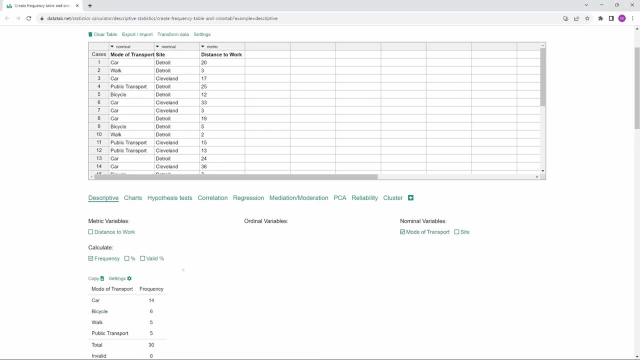 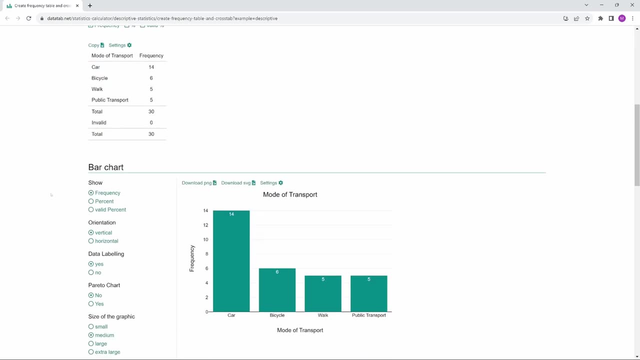 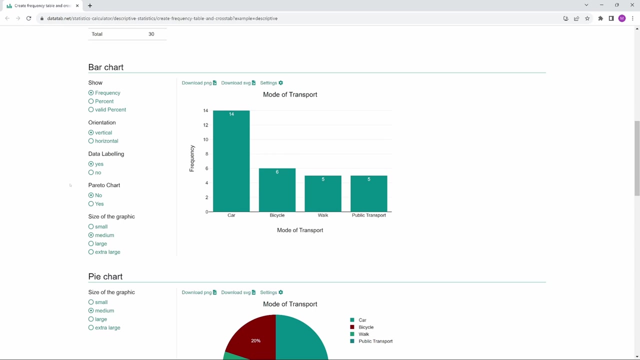 here Now. if we only click on mode of transport, we get a frequency table and we can also display the percentage values. If we scroll down, we get a bar chart and a pie chart. Here on the left we can adjust further settings. 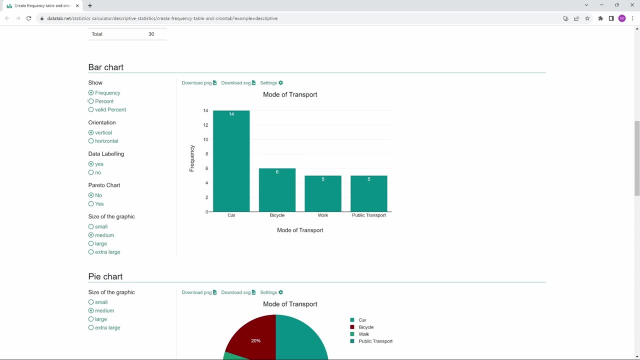 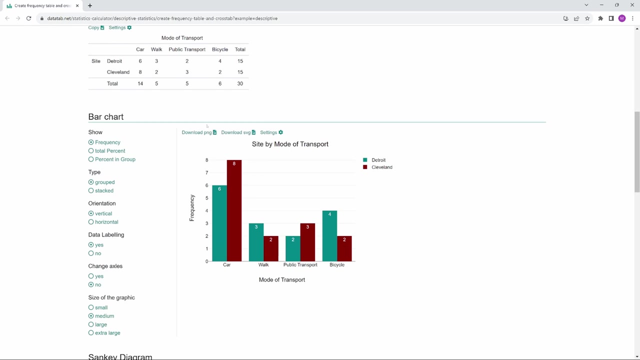 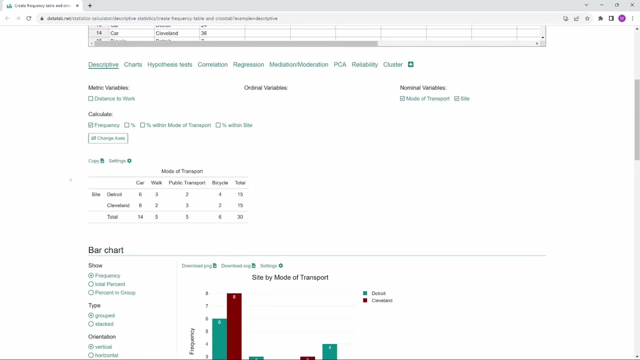 For example, we can specify whether we want to display the frequencies or the percentage values, or whether the bars should be vertical or horizontal. If we also select site, we get a cross table here and a grouped bar chart for the diagrams. Here we can specify whether we want the chart to be grouped or stacked. 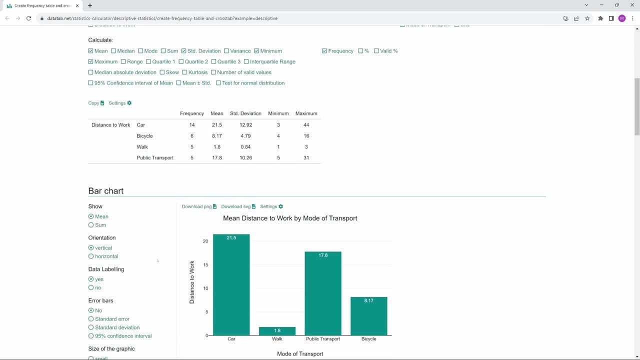 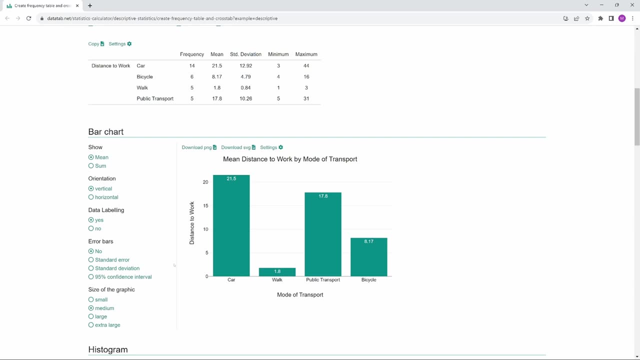 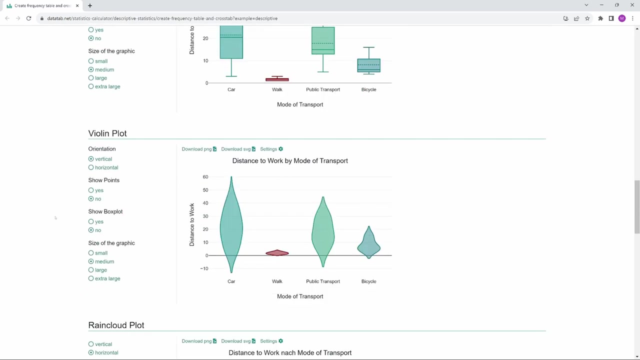 Okay, If we click on distance to work and mode of transport, we get a bar chart where the height of the bar shows the mean value of the individual groups. Here we can also display the dispersion. We also get a histogram, a box plot, a violin plot and a rainbow plot.